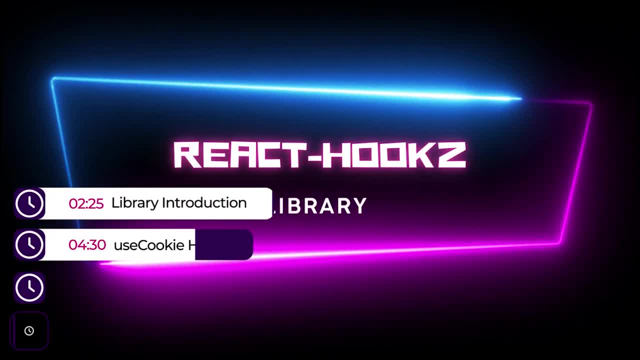 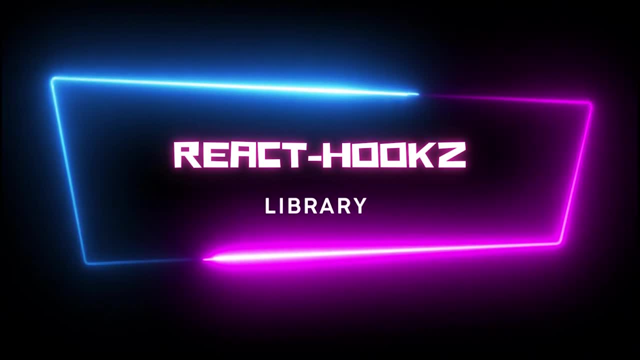 Hey guys, how's it going? I'm back here with another video and today I decided to bring this video where I'm going to be introducing to you guys one of my favorite libraries in React. This library I actually found out just a couple weeks ago, but immediately when I looked at it, I took 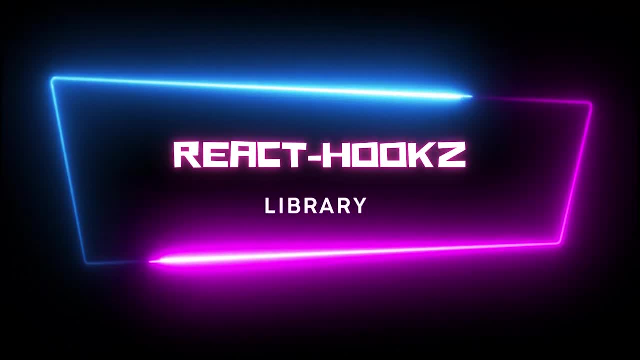 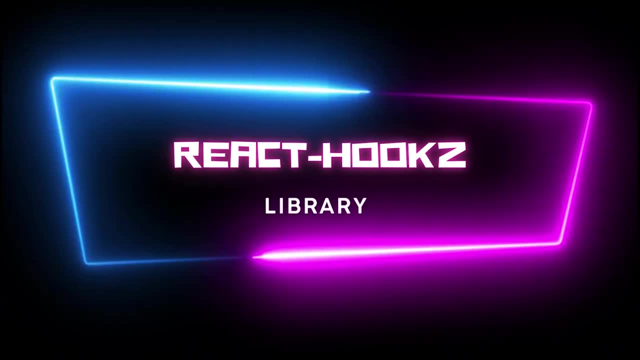 a look at the documentation and I found it pretty cool, So I tried it out and I have been using it ever since. Now, before anyone says anything, this video is not sponsored by this library. I have no affiliation with this library. I actually just found it kind of cool and it's good that I don't. 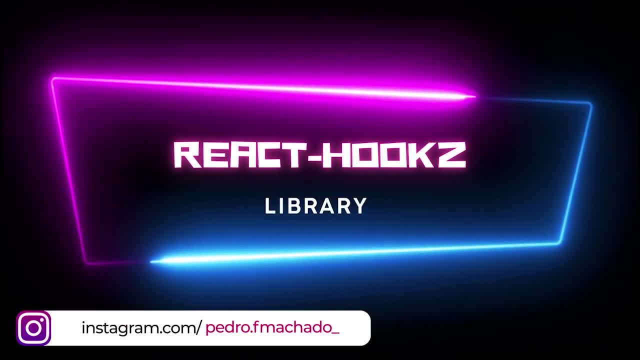 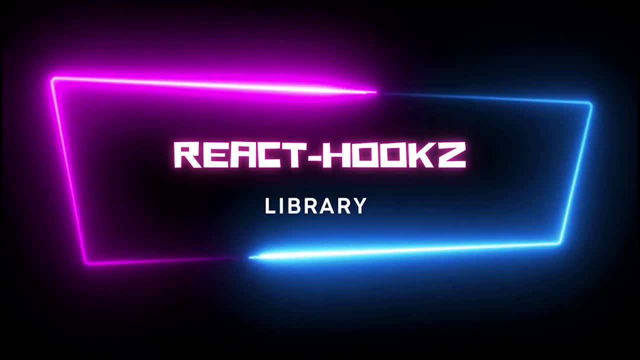 have any affiliation, in case this library is not well maintained in the future or the developers do something to it. I don't want to be responsible for the actions of the library that I have nothing to do with, but I do think it is really cool at the state of which it is right now. Now I'm talking. 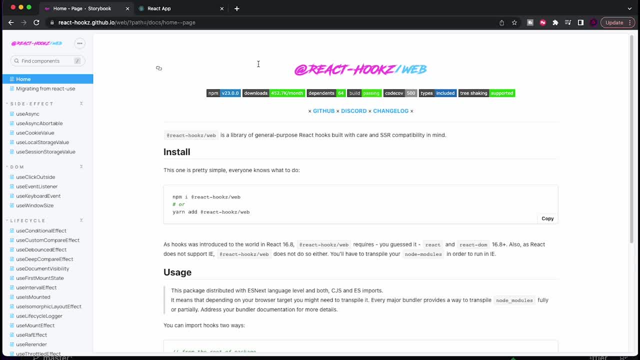 about the React Hooks Web Library. This is an actual update from the React Use Library- You can see it over here- which is a library that basically its main purpose is to contain a huge amount of hooks that could be really useful inside of a library. So I'm going to show you guys a little. 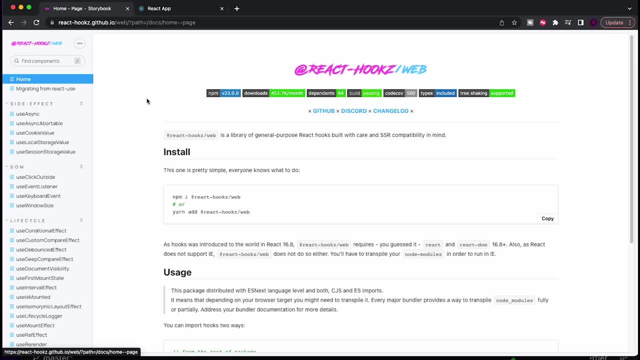 bit about the React Library. Now I know what a lot of people are saying, like, if you're going to deal with hooks, why not just create your own whenever you reach the necessity for some sort of hook? Well, because this library can be really cool in situations where you don't have that much. 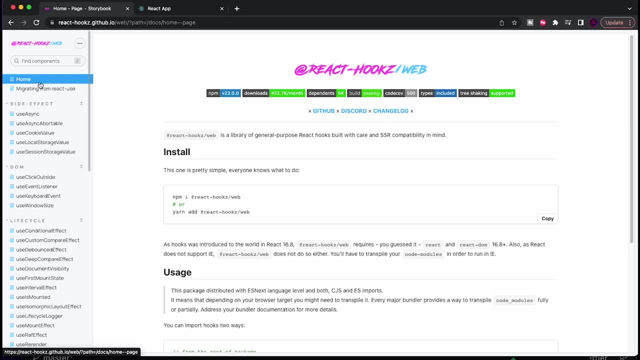 time, or you don't want to spend that much time just creating all of the custom hooks that you might want in a project. For example, I always find myself needing to create a debouncer hook or some sort of hook that is going to be used to fetch data, Or if I'm working with something more. 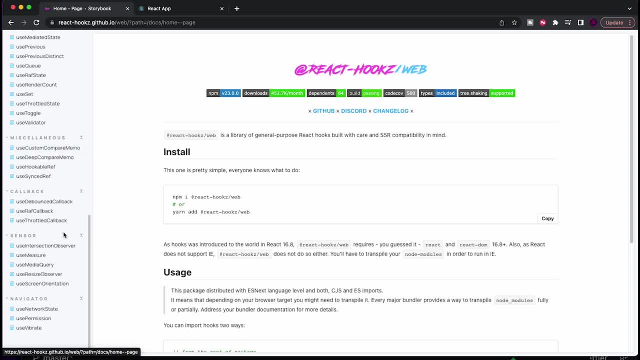 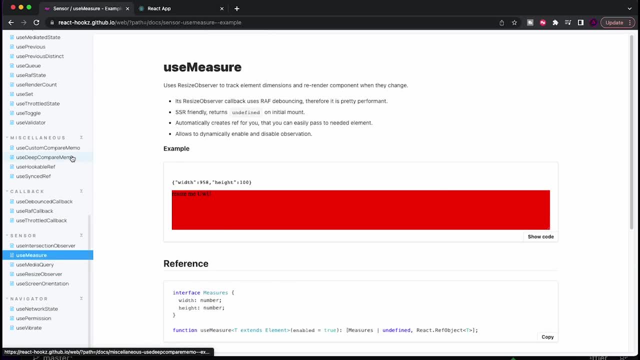 complex, like a UI that requires me to know the size of my screen. something like a use screen orientation or a use measure could be really cool, right, But I find it annoying that I have to remake them every single time, And obviously I could just copy and paste from my own previous. 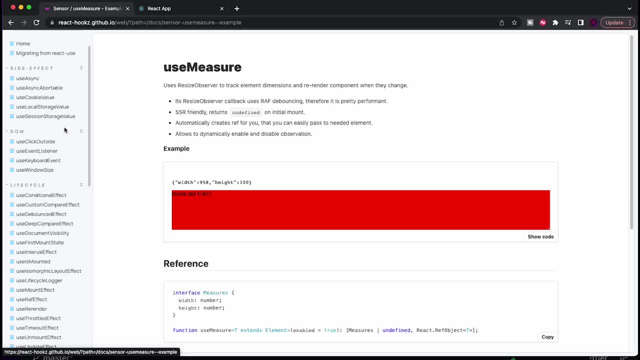 projects, But I feel like in some situations, it could be cool to just have this library of pre-made hooks available for you, especially because there's a lot of hooks that could be used to solve situations that you're not even aware they exist, So I wanted to introduce you. 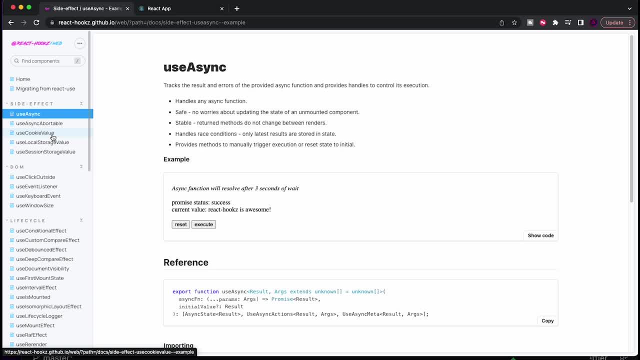 to this library because I know a lot of you guys might not know it yet. So, before we get into the video, if you could leave a like and subscribe, I would massively appreciate it. We're getting back and posting a lot of videos every single week, So I would really appreciate if you guys could. 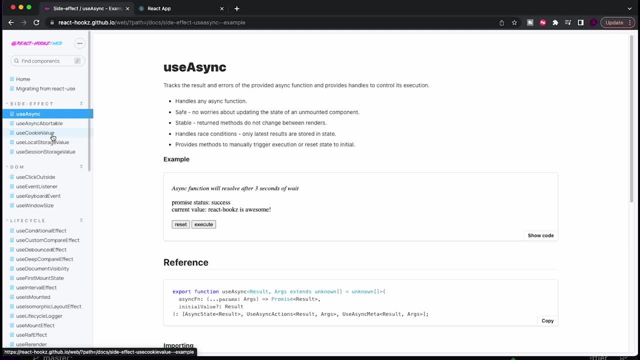 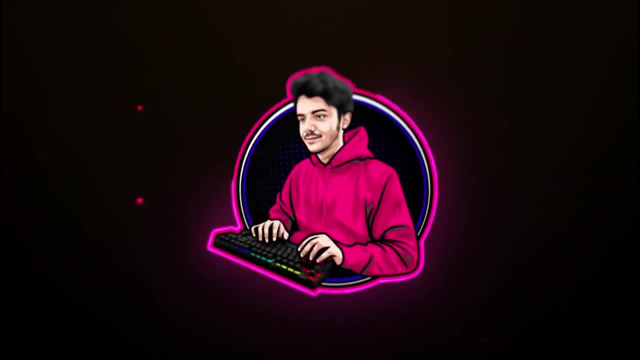 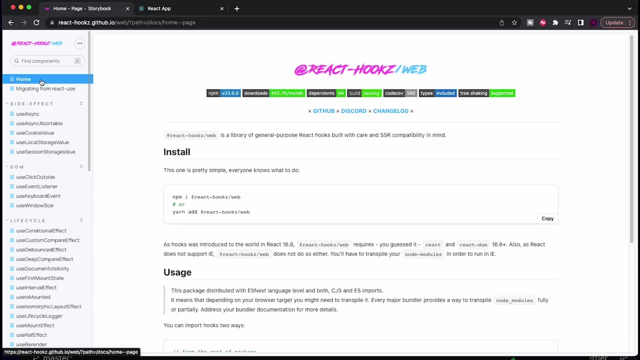 leave a like and subscribe. That would really help push my videos to more people. And yeah, that's basically it. Let's get into the video, Okay, everyone. So, like I said, this video is about the React Hooks web library And I want to start out by just talking a little. 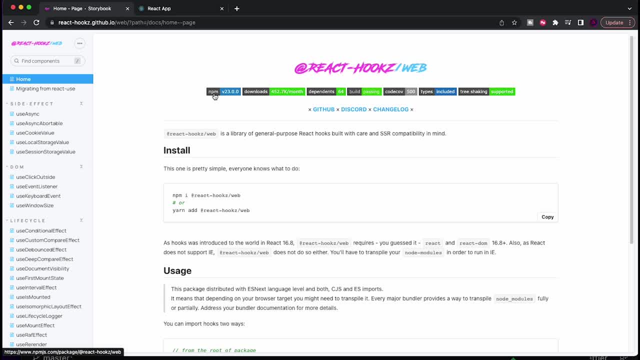 bit about this library. It is, like I said, a hooks library completely compatible with the newest versions of React. It is a library that is used a good amount. actually, It's not something that is used like. it's not one of the most used libraries in the world, but over 100,000 downloads. 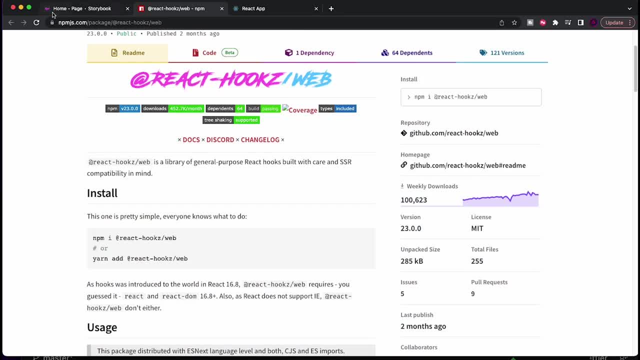 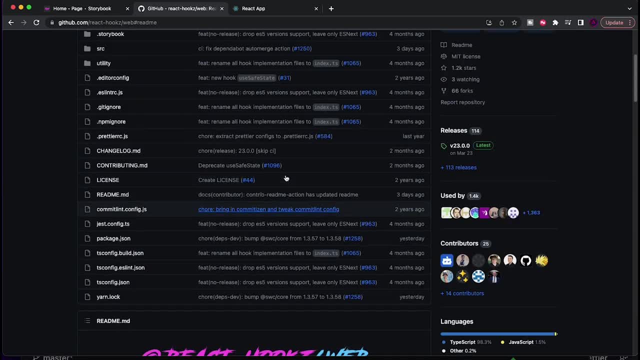 per week is a pretty good number in NPM And I do think that it's well maintained. I took a look at this library, I took a look at what they're working in And it seems that some of the changes like were three days ago. Some of the changes were a couple months ago. It seems like there is a team. 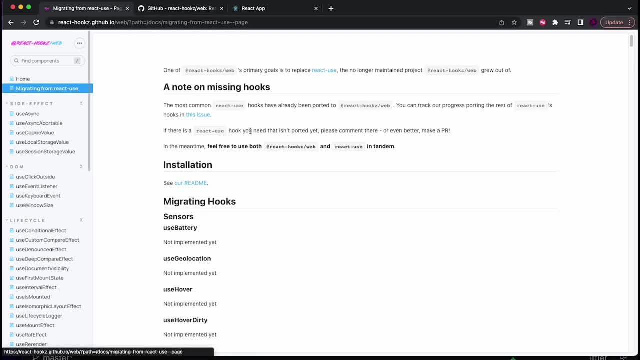 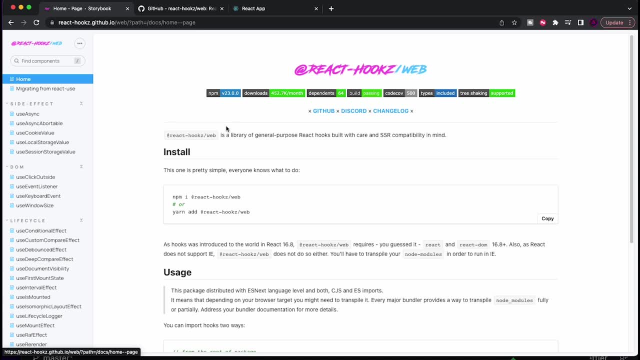 behind it, And the main purpose why they migrated this from their previous library was exactly because it was no longer maintainable. So I do believe that this library will be something that will continue existing And I would trust to put this in your project. So one of the main things: 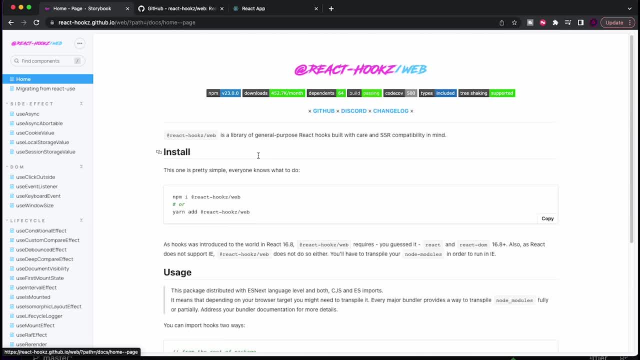 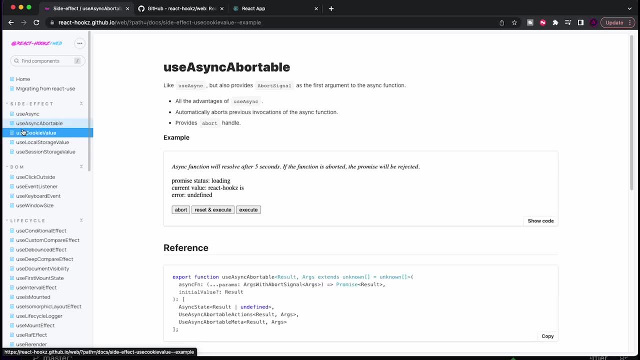 that I like about this library compared to any other hooks library- which, by the way, there's a lot out there and you might know this- is the fact that the documentation is amazing, Like if you go through each of these documentations over here, you would see that. for 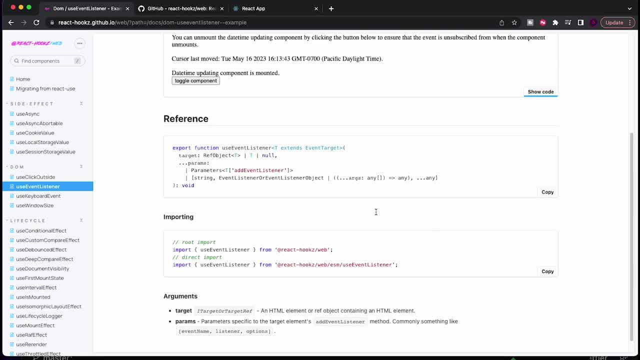 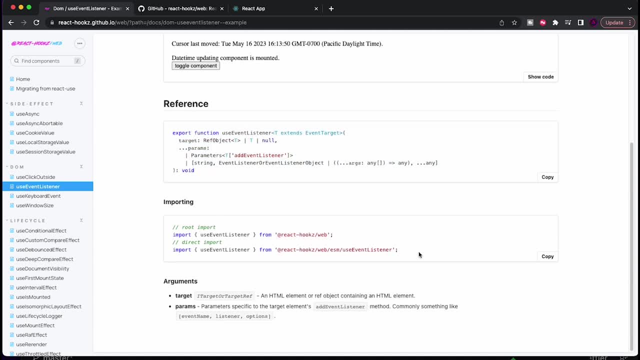 each hook. there's like an example. you can see the code they used in that example. There's also references to how to work, data types and everything related to each individual hook and how to import them. There's also a clear, detailed explanation of each arguments that the hooks can take and some 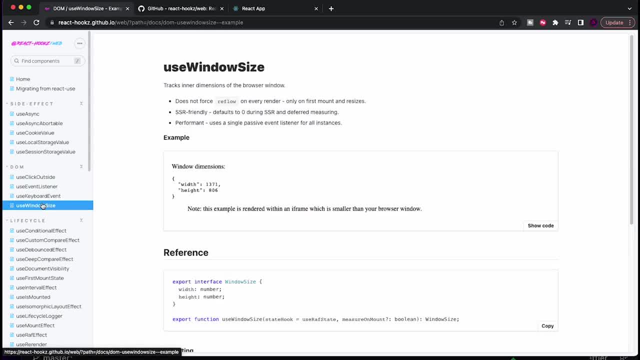 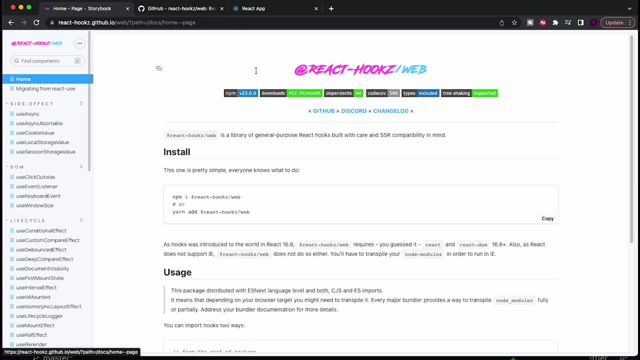 stuff related to how it works. So it is pretty good- the documentation And also I forgot to mention, but as you can see over here, this is compatible with TypeScript. They included types, as said over here, right, So the documentation. 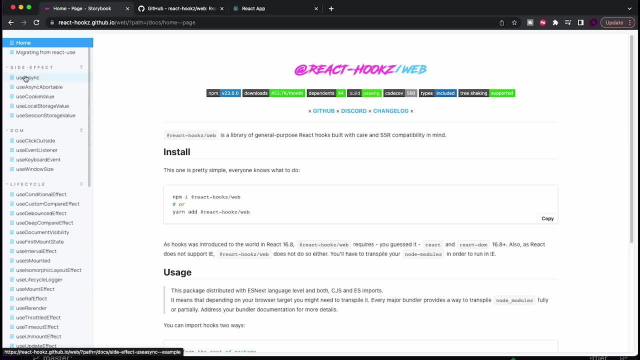 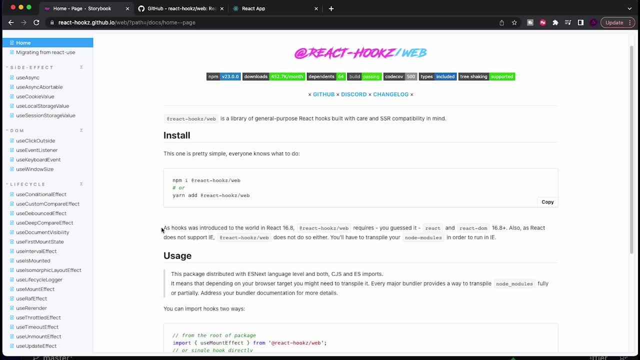 is amazing. And also the second thing is that it has a lot of hooks, which you might expect the bundle size to be, that to be big, But to be honest I don't think it is that big compared to other libraries out there that might introduce even less features in this one over here. So the amount of 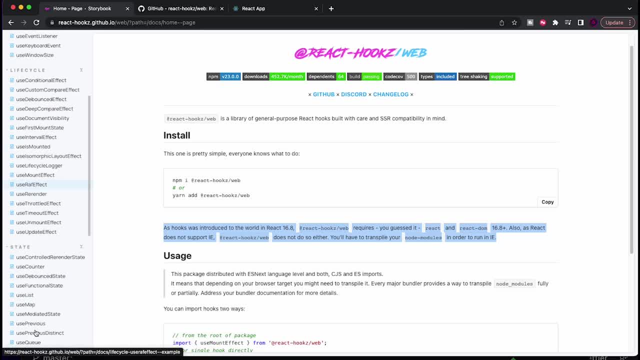 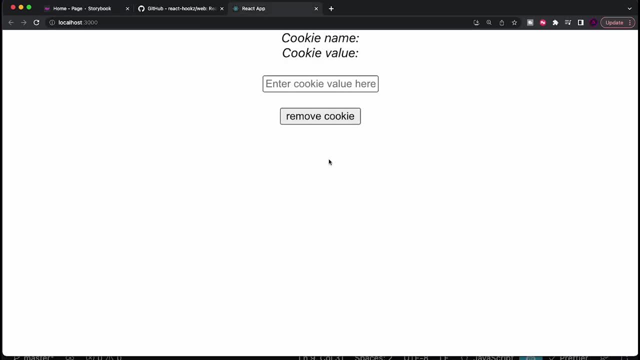 hooks that they have is ginormous, as you can see over here. they have for any kind of situations and I actually selected a couple that I wanted to show you guys How to use. that I found really cool. Okay, so the first hook I want to introduce you guys is the use. 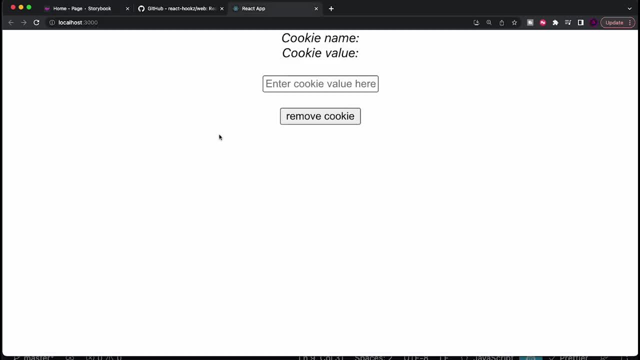 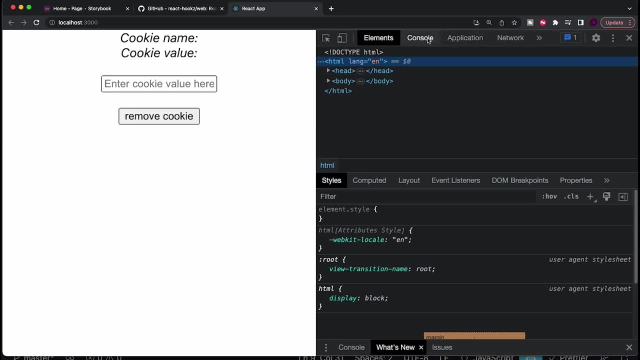 cookie hook. I believe it's you use cookie value. The reason why I want to introduce this is because I personally know that, especially for beginners, it's kind of hard to do with cookies in JavaScript in general And it's nice to have a hook that could facilitate that, And I was recently using I. 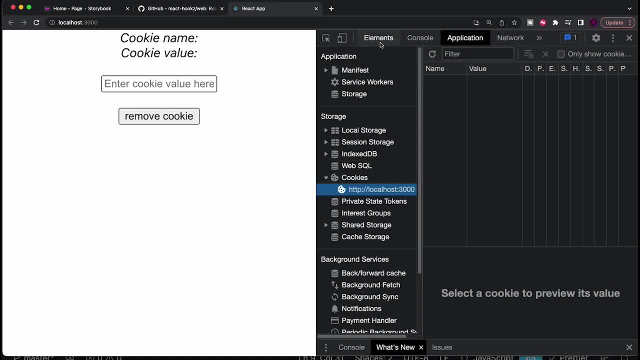 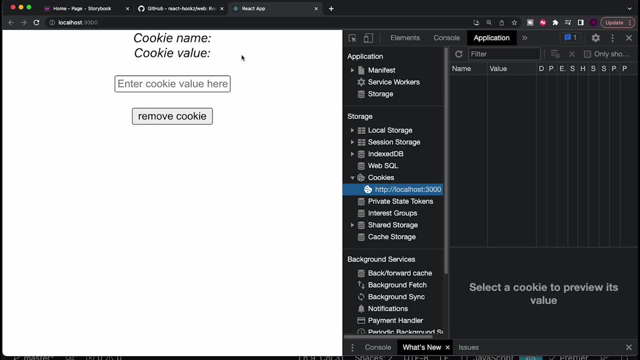 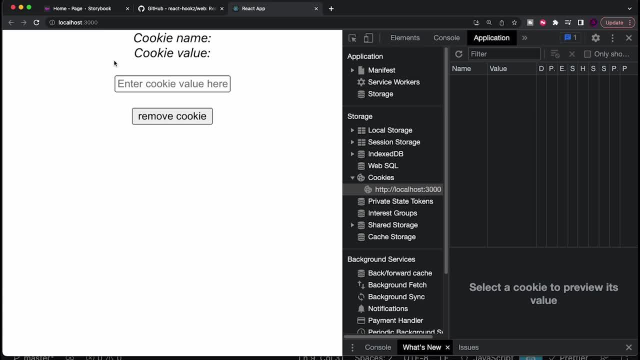 So I wanted to show you guys how to use that one. So you see, over here we have this simple example where we have this input, And what I want is, whenever I type anything over here, it will automatically set it into a cookie And we can find it in our applications inside of our browser. 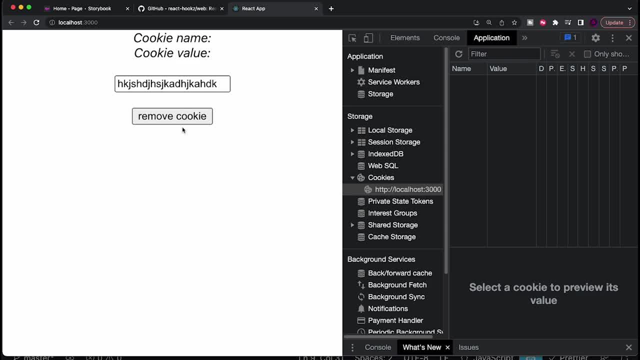 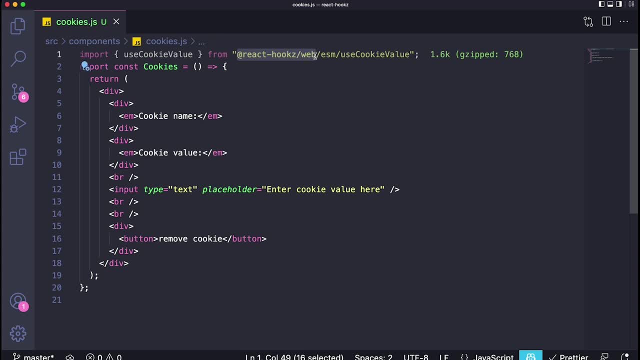 right, And if I click on this button, it should remove the cookie. Now, how easy is it to implement that using this library? Well, the first thing you would have to do is, obviously I would recommend installing at react hooks slash web. this is the main, main core library And they have individual imports if you want to. 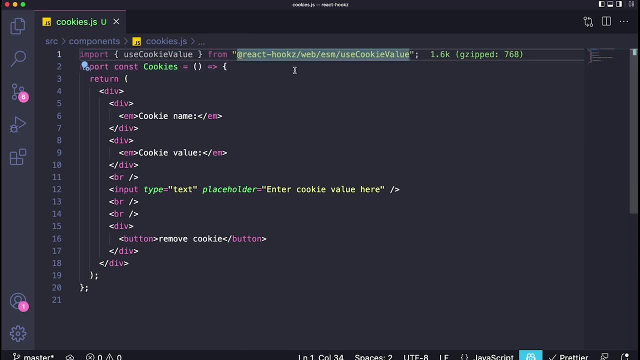 by just grabbing them like this. But the thing is, with with this specific hook, a couple of the hooks that they have might require you to install an extra library or an extra dependency. That's depending on you If you want to do that. I found the cookie hook kind of cool, So I knew that it. 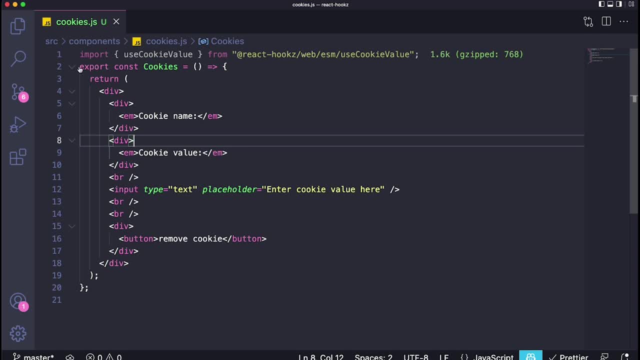 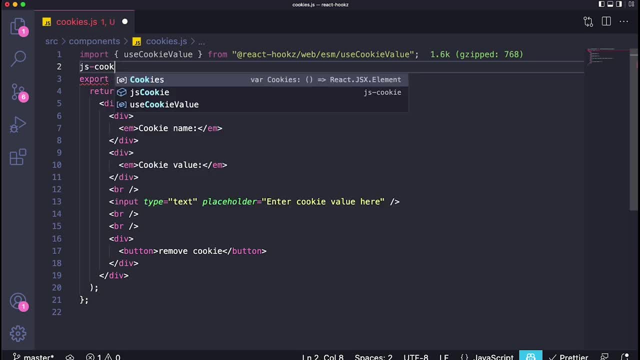 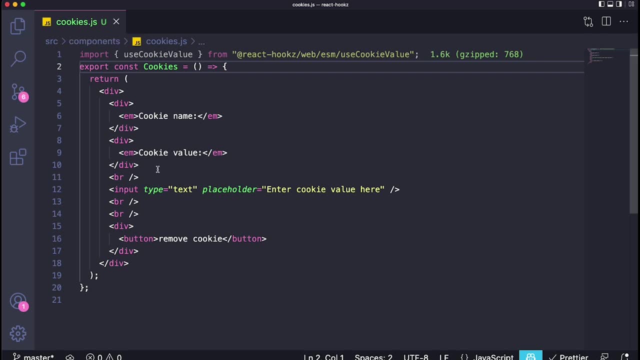 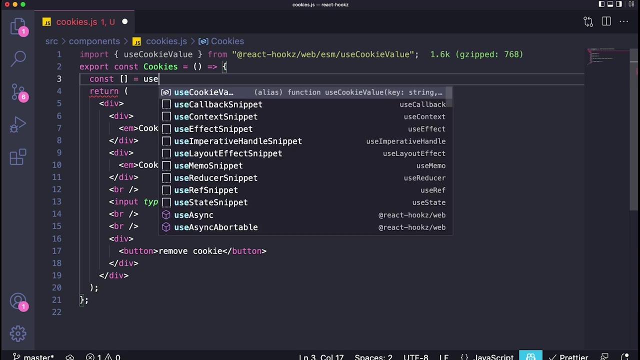 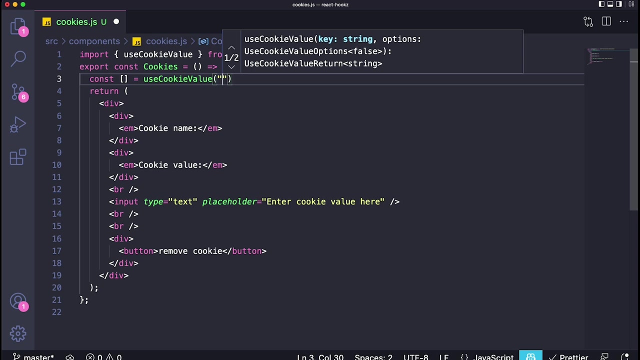 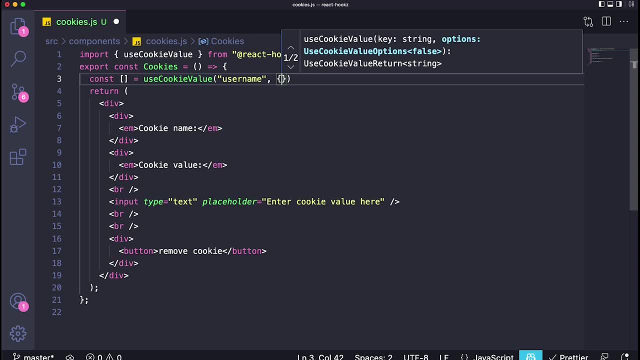 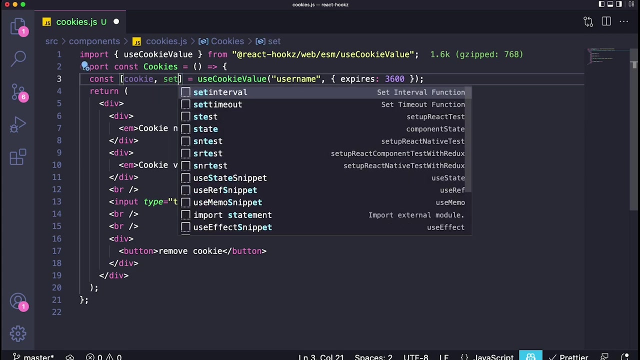 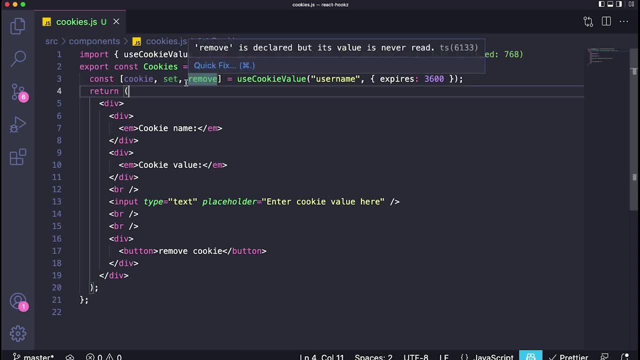 create and to update and to delete a cookie. so, for example, over here, if you want to, whenever we type on this input to actually set the cookie to the value of the input, all we have to do is say on change, then just grab the value of the the cookie by saying event and just say set event. 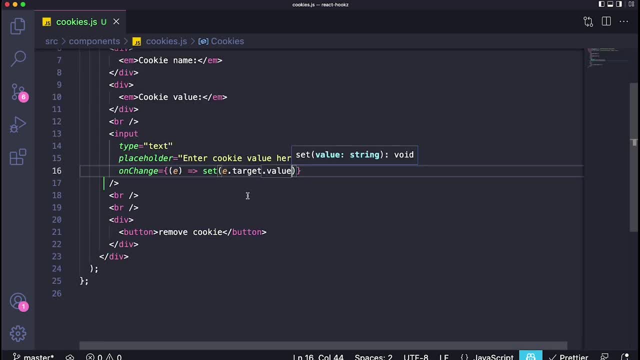 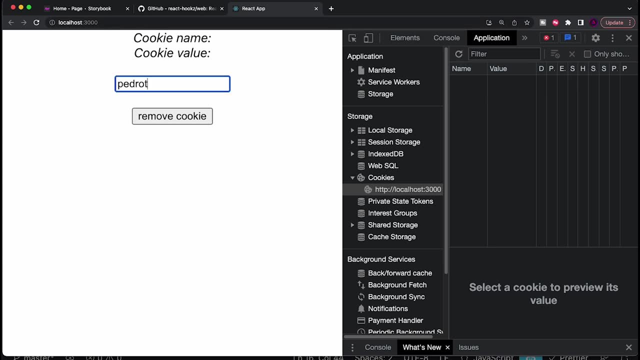 dot target dot value- then you'll see that uh over here. uh, if we're refreshing, right, there's no over here. but if i type something like pedro tech and i refresh this, now we have a cookie with a username as the name and the value would be pedro tech. if i delete this, just delete even. 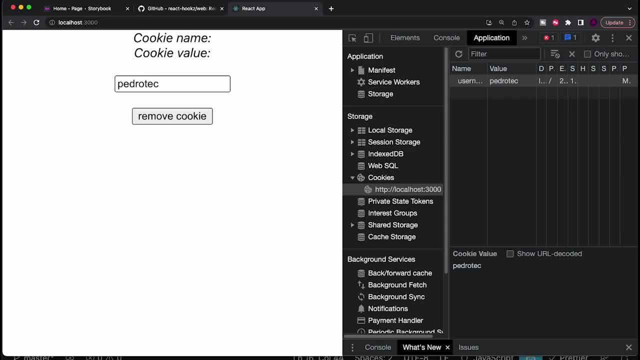 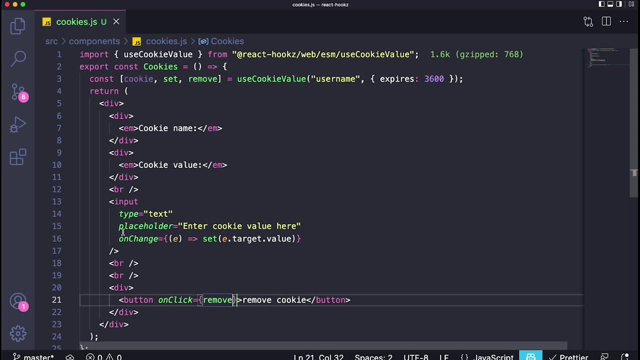 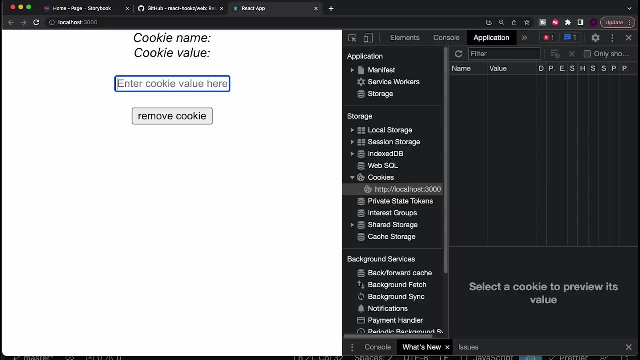 one of them. you see it constantly updates. now, if i want to remove the cookie, all i have to do is just add an on click to this and just call the remove function. as simple as that. you'll see that if i click on this now, the cookie was removed, and also if i want to display the cookie all. 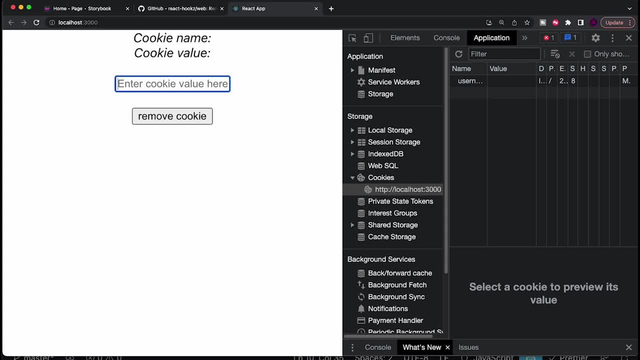 i have to do is just add an on click to this and just call the remove function. you have to do is just display the variable cookie, just like this, and you'll see that if i type pedro tech, as it's updating over here, it's also, uh, displaying the value of the cookie over here. 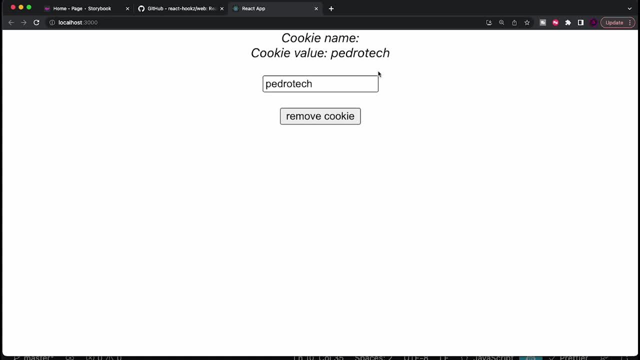 and it works pretty well. so in my opinion, this is a really cool hook. it's one of the- it's great example of how simple this library makes their their hooks look like, and if you check out the documentation, you'll see that it might even be better than my explanation, right. 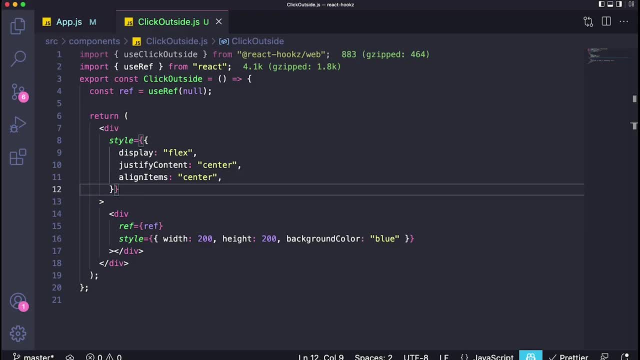 now, that's how good the documentation actually is, okay. so the second hook that i want to show to you guys is the use click outside hook, and this one is actually pretty cool because i found myself in situations where i had to create something either similar or exactly the same. 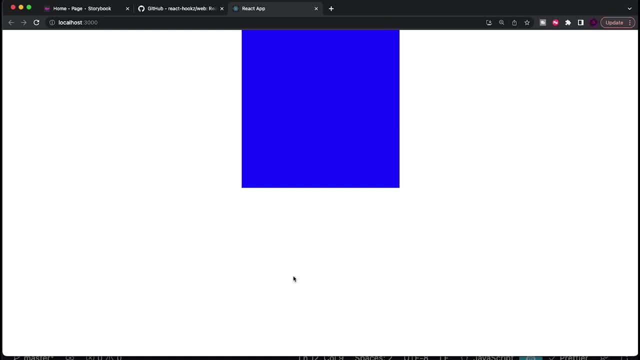 as this hook. so imagine we have some sort of website which requires us to detect if we're clicking outside of a specific dom element. in this case, let's try to detect if we're clicking outside of this blue square right. as of right now, this is not happening. we are not detecting any. 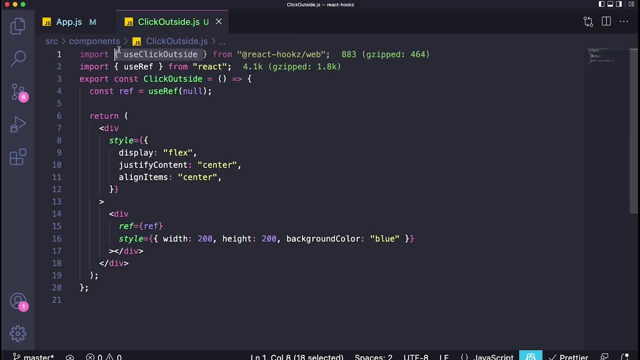 kind of way, but with the use click outside hook. and, by the way, with this one you don't have to install any actual libraries. uh, like we had to do with the cookie one. actually, the cookie one is the only one that i found that you had to do that, so that's not a common occurrence. um, so with 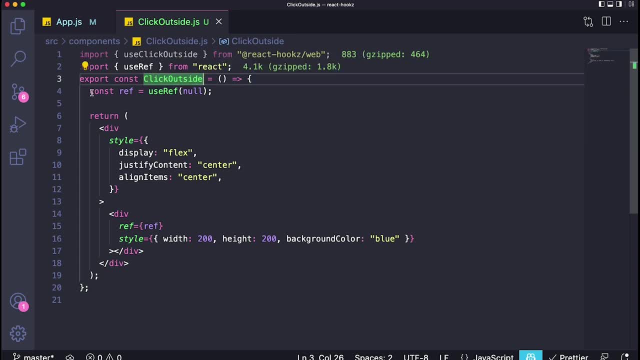 the use click outside. all you have to do is you first have to set a ref uh to the div that you want to know if you're clicking outside of right. so i created this div, made it blue and made it have a width of 200 and a height of 200, and i've set the ref to be equal to that, and then we're. 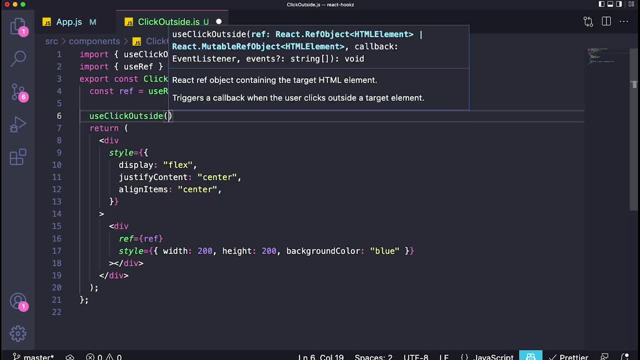 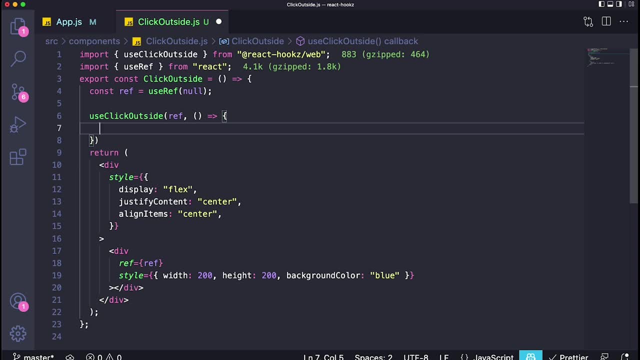 going to use that ref and call the use click outside hook and just pass the ref like this. then you will have a callback function which, um, inside of here we can just write whatever action we want to execute when it is clicked outside, this function, this hook, will handle everything for us. uh, all the logic for detecting if it is clicking inside. 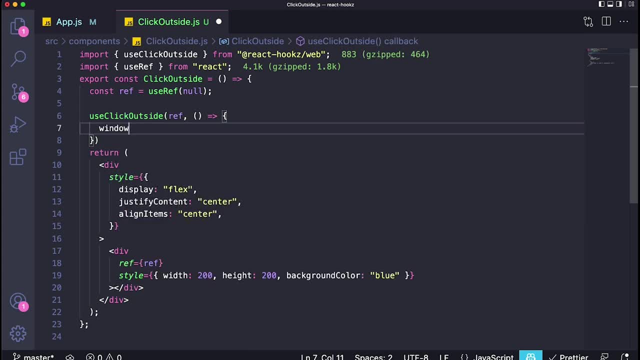 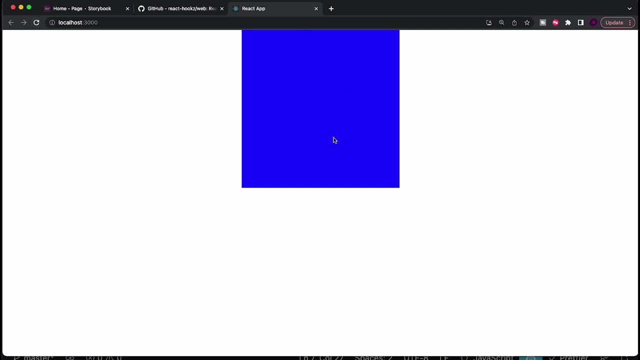 of this reference or not. so we'll just put over here that we want a window dot alert. actually just say alert, just like this, and say clicked outside and let's see if that will work. uh, obviously it will. we're clicking inside of the, the blue square, nothing's happening. but if i click, 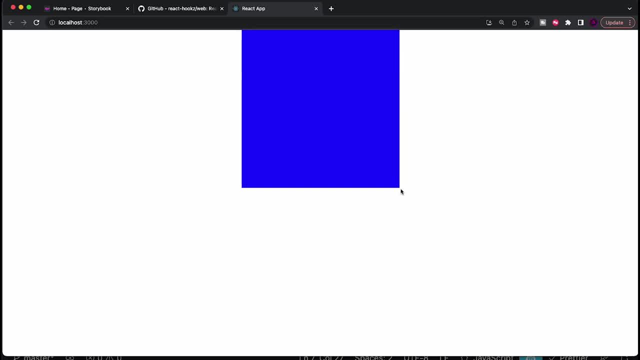 over here. it detected that i clicked outside. even if i try to click as close as possible, it was a little bit outside. but here it isn't right. you can see, it literally detects if it is outside. so this is a pretty cool hook. i think it has a lot of use cases. but you guys are the judge of it, i'm just 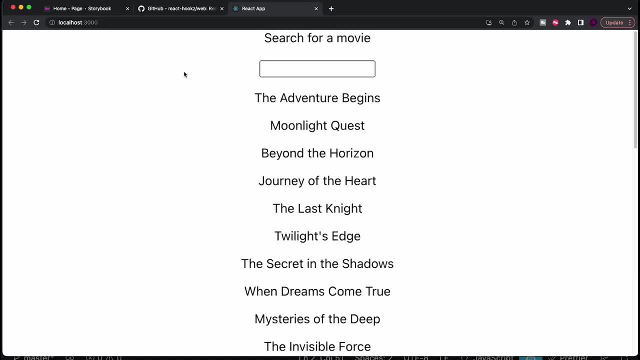 here demonstrating the ones that i found the coolest. now, this last one is probably the most useful, in my opinion, because, uh, we've all needed to deal with a debug answer when working in projects, because the concept of debouncing allows us to limit the number of times a function or an action is called, which improves not only performance in a website. 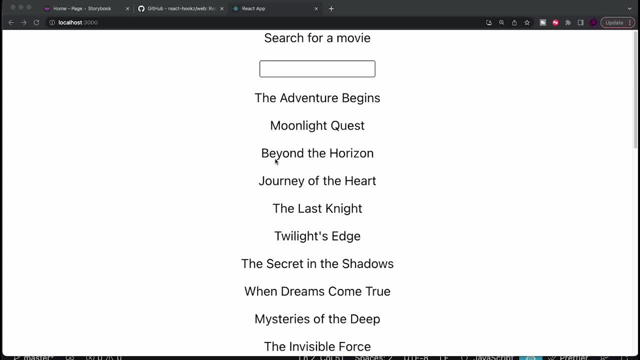 but also improves the user experience. the most common example of debouncing being used, in my opinion, is whenever you're trying to fire a lot of actions in an input as quickly as possible, you don't want a function that is dealt when you change that input to be fired. 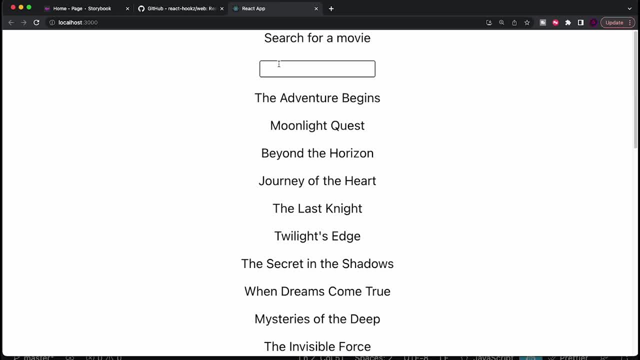 a bunch of times, because maybe a user is typing it so fast that it takes longer to to to execute that action than to, uh, complete the action that the user is doing. so what i mean by that is, imagine you have, um, a list right or a search bar, and this is not the example that i'm talking about, right. 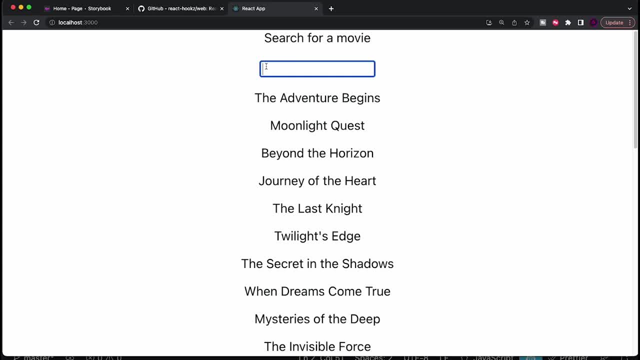 now this example is actually. i'll explain in a bit. so imagine you have a search bar and whenever you type on the search bar, without even pressing enter or clicking on a button, it will automatically search for, make an API request to an API and search for something right. so this is really commonly seen in stuff like 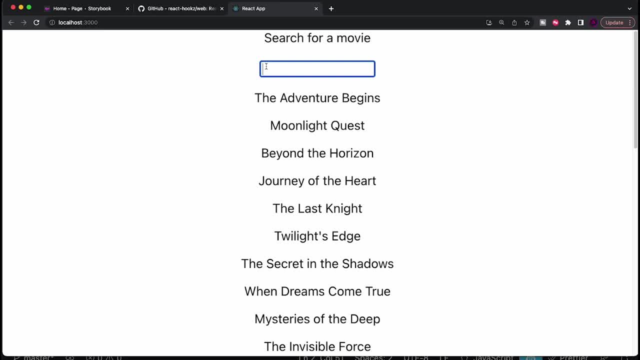 uh, Instagram or Netflix, when you're searching for a movie, it will give you. it will try to filter out for the options as you type right now. imagine if you were searching it really fast, then maybe before the API request is done to search for a movie, you are you actually typed another letter. 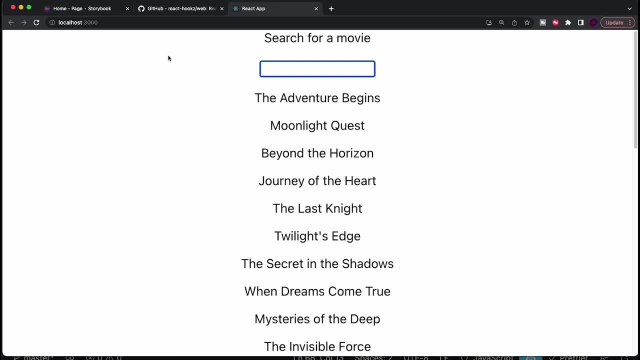 so that request uh is invalid or does it doesn't make any sense, right? an example, without actually making an API request is, with this list over here, what it's doing? uh, it's basically, whenever there's a list of movies, right, a big list of movies, and as 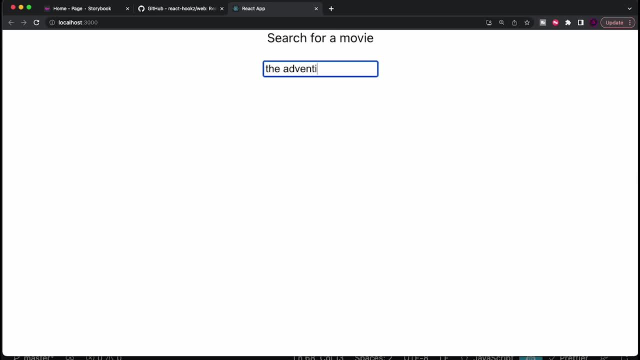 i type it will actually filter out for the movies that, uh, the list or the search bar is searching for. now, imagine i get to this point over here. there's a bunch of movies that includes the word duh, but no movies include the word the right now, if i'm not using a debouncer, i'll, i can just keep. 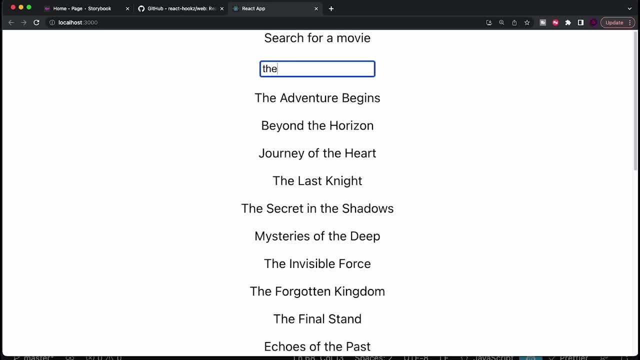 deleting and opening, and you see, it happens. the search, the filtering happens immediately, right when the search is uh, done in in linear time and just in a small set of data like this one over here. but if you're making an API request, it definitely won't be fast enough to be able to. 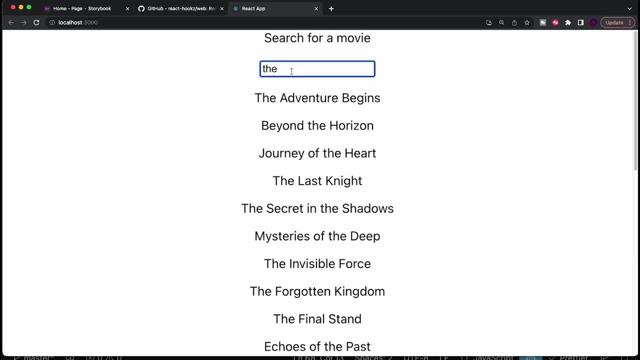 complete before the user types the next character. so you need to add some sort of devouncer that will allow you to limit the number of times you're making that request and wait a little bit before actually making the request. so we'll actually implement that by using this uh library's version. 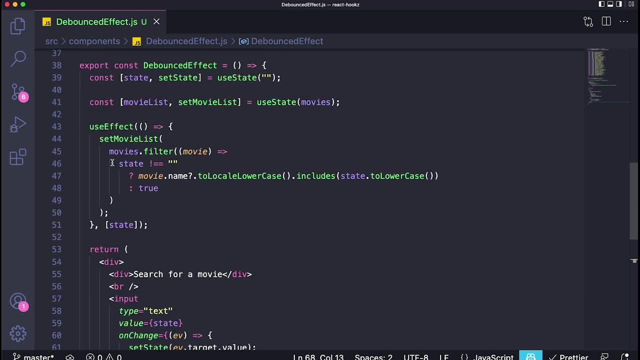 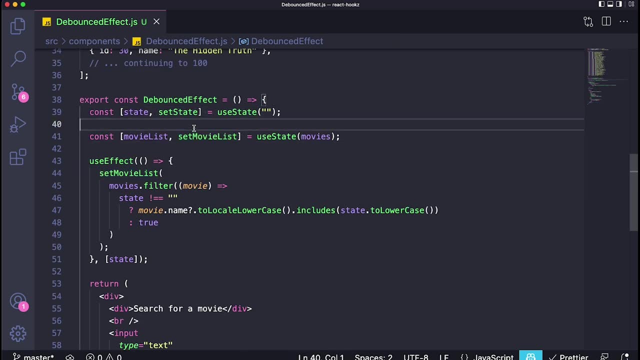 of uh, the bouncer. so uh, as of right now, the code is simply like this: i have a list of movies. i have a state called state, which is just for what you're searching for in the movie, and a state called movie list, which is just a list of movie, and whenever the state value changes, so whenever. 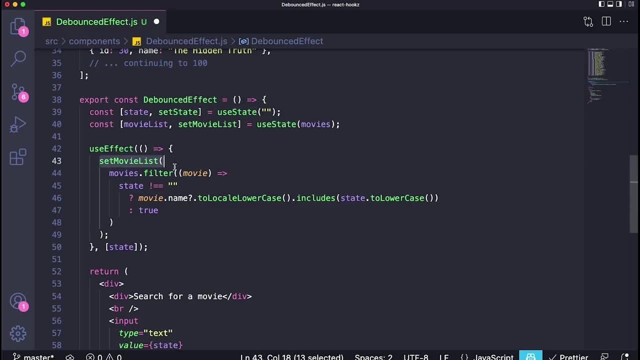 you type on the input. all it's doing is it's just updating the movie list to be a version of itself, but without the movies um that are not like. that doesn't correlate to what you're typing in the search bar. if you're interested in checking this out, i do have videos on the search bar. 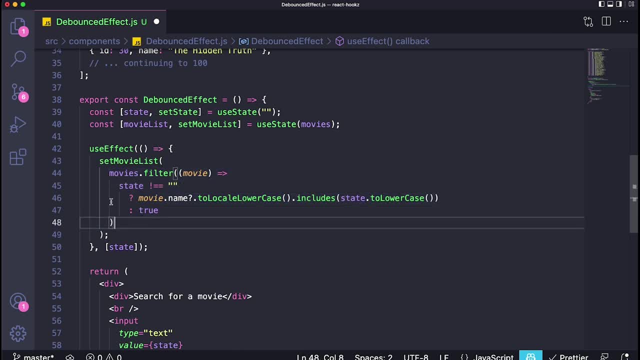 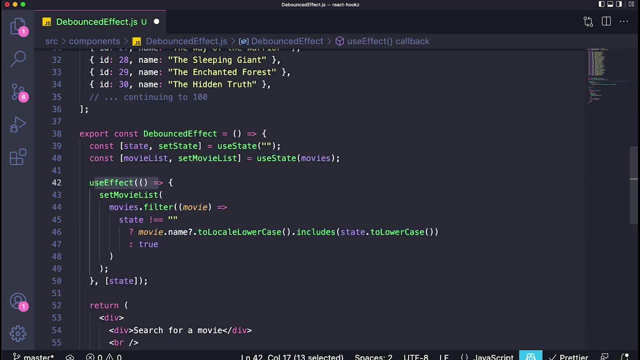 search filters in react and inputs. i have a video explaining all of this, so if you're interested, go check that out. but the important thing here is that whenever the state is changed, the use effect it's called so immediately. when we type a new character, this is done, but we don't want that. 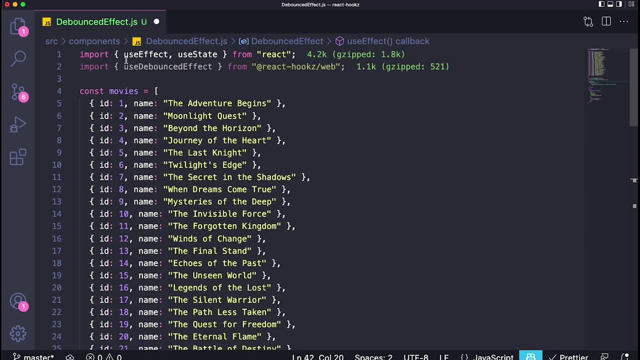 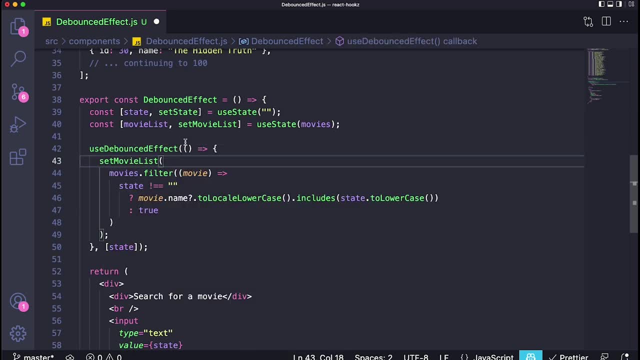 right, we want to use a debouncer. so the way we would do this is by actually using this use the bounced effect hook and replacing the use effect by that. so i'll say: use the bounced effect. so over here we're actually going to have a state as a comma. 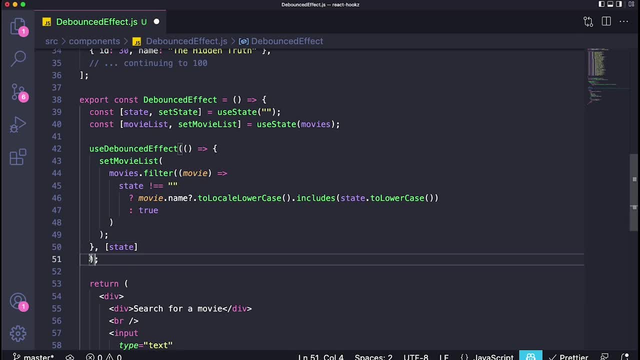 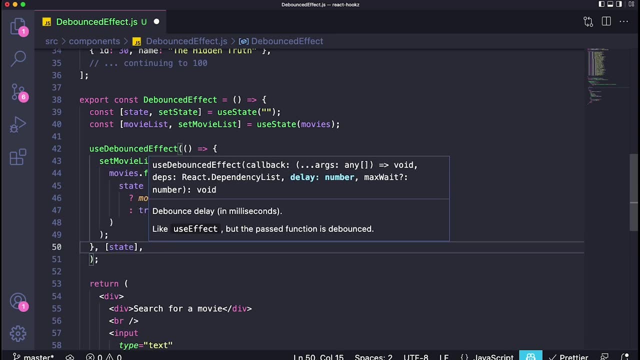 like this, but also put in some pieces of information. so the first piece of information we want to put is um, the delay that we want to add to our debouncers, so obviously this will be milliseconds, so this just means that we want to wait a certain amount of time before executing. 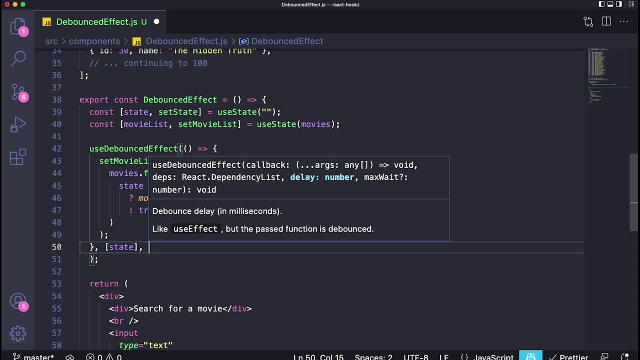 this action again. it's basically running and as the state changes, but with a small interval. so over here we're going to put a delay of around 200 milliseconds, similar to, i think, what they did in their documentation, and then, finally, we want to put in a delay of around 200 milliseconds. 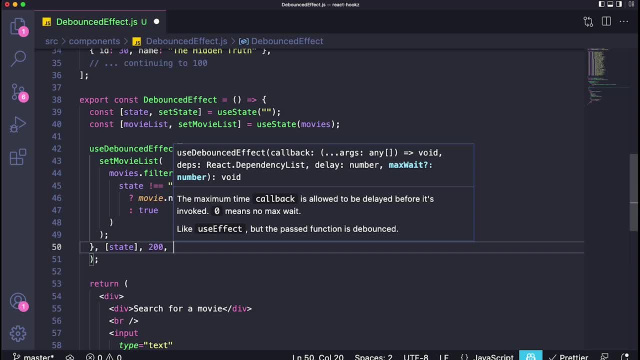 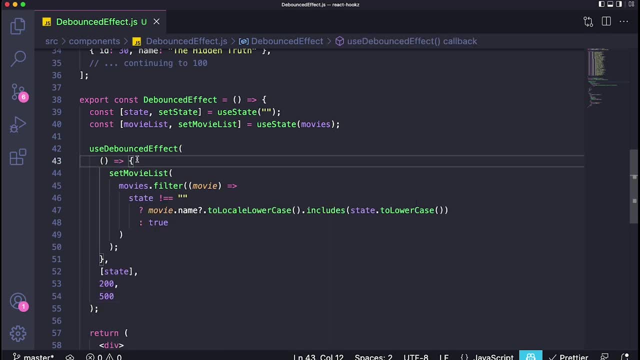 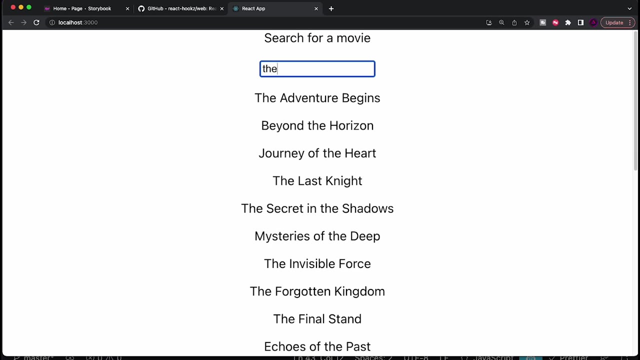 so the maximum amount of time that the callback is allowed to be delayed before it is invoked. so i will just follow what they also put in the documentation, which is 500 and uh, let's see how it looks now. so if we do this now when i start typing, right, it does take a bit to to actually 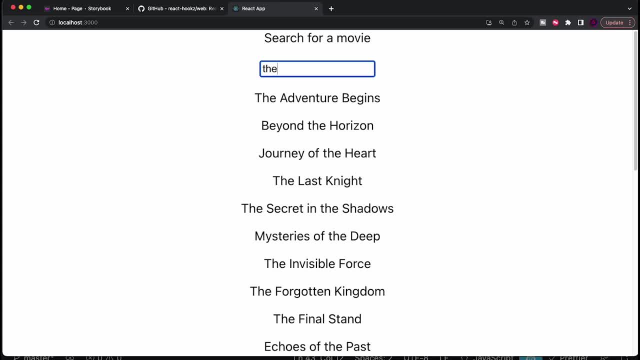 run, but it's not that bad as a of a user experience, actually better because it does seem a little bit delayed, but also it doesn't have that immediate flash of ui change like it was before. the best example is if i type the e a bunch of times, sometimes it doesn't even change. see, because 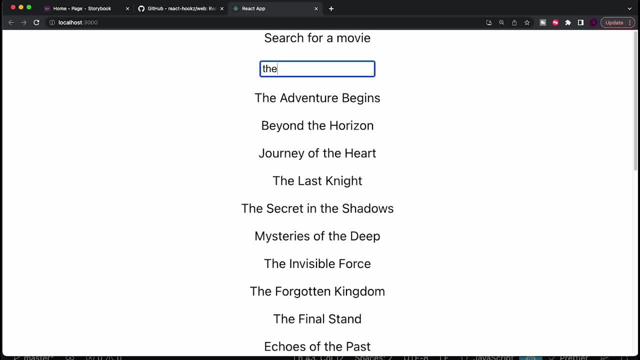 i'm firing a tick as quick as possible. obviously it will change after like 200 milliseconds, but that's expected because i am searching for other stuff right. so this is the use- the bouncer effect- and it's a pretty cool hook in my opinion and i do like the way they implement it. you can check it. 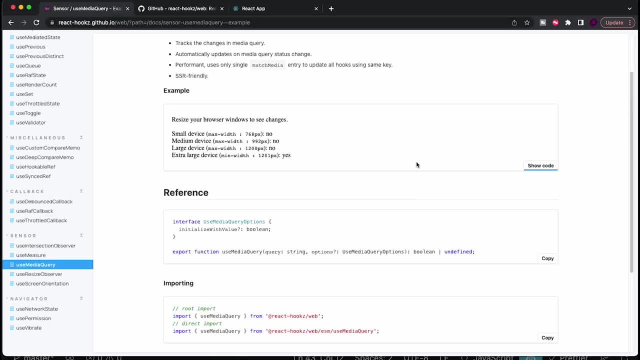 out in their documentation as well. now, those were the three hooks that i wanted to like manually introduce to you guys, but i want to shout out to a couple ones that i found cool as well. i really like the way they implemented it, and i'm going to show you how to do that in a second. so let's. 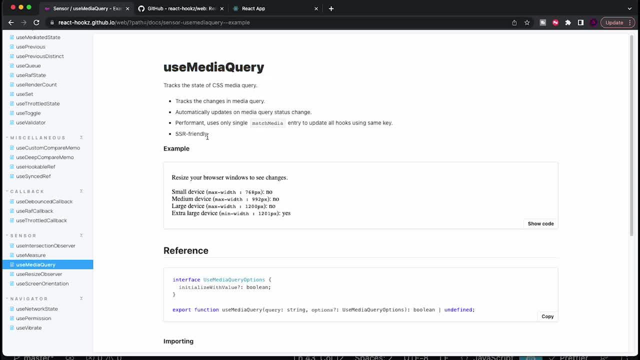 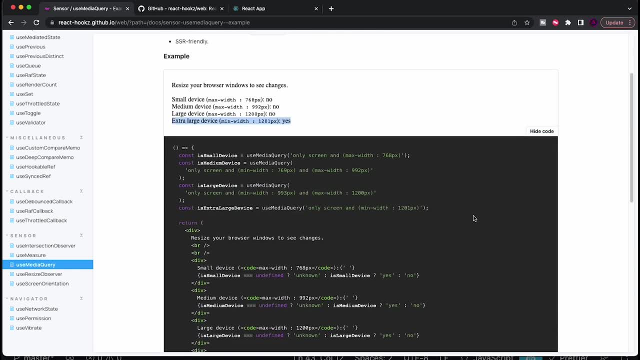 start with the use media query, because it is nice to be able to track css media queries without being css. it gives you the actual css media queries but in your actual react code. so if you want to use conditional logic to do something related to that, you can do. um. so like imagine, 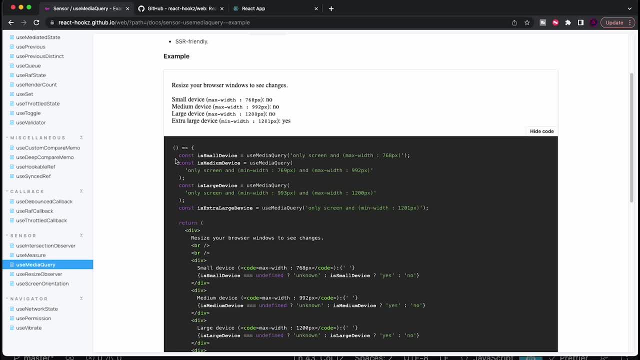 you can build a website that contains, um, some sort of functionality if it's, uh, if the screen is smaller, and it doesn't if the screen is bigger, right, that's just one example of a use case that you could do. also, it is really easy to use the css media query to track css media queries without 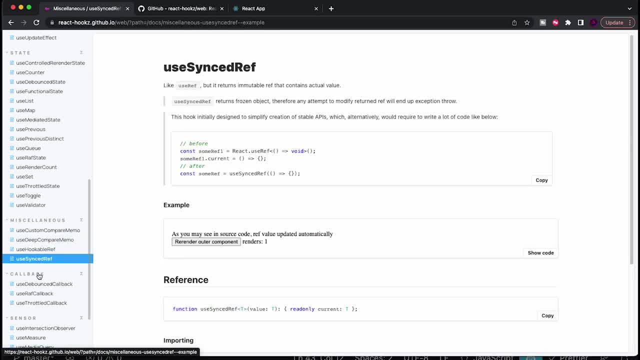 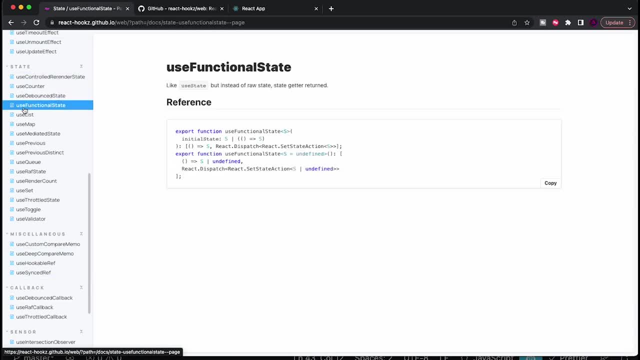 being css. it's really cool that they have a bunch of like good hooks for performance, as you can see over here. a lot of them could be used for that purpose, and also there's a lot of hooks that can replace individual data structures. so you have the use list, you have the use map, the use queue. 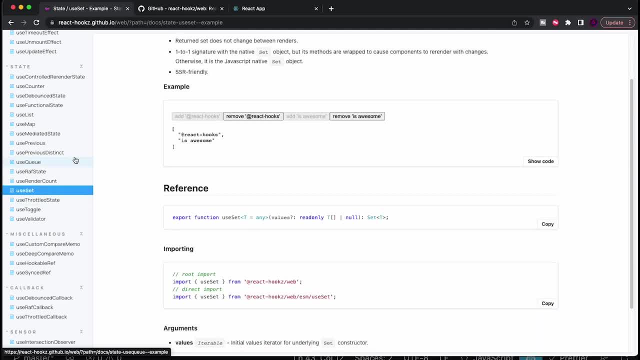 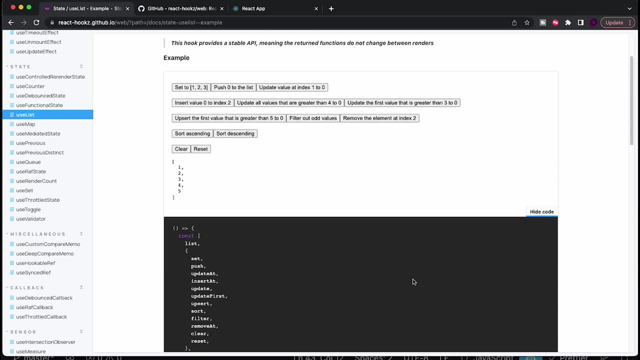 the use set. now why you might want to use that. well, because, for example, the use list is the most simple example here. when you have a list, there's a bunch of built-in functions that you can call from that list. but it would be cool sometimes to just have a hook where you define the list that. 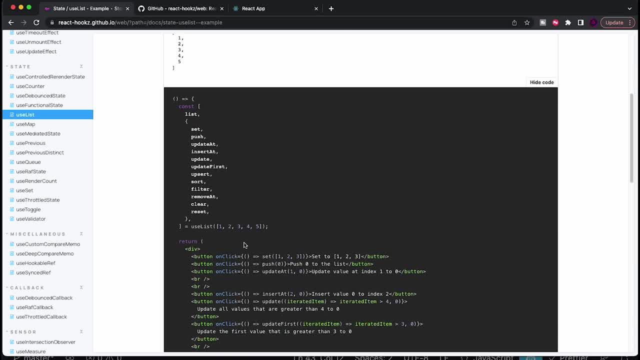 you want to deal with and then you just have individual functions. they can just call, like: if I want to push something to this list, I don't have to grab its name and say dot push, I can just use the push function. if I want to update, I can just do this filter- same thing. there's a lot of functions. 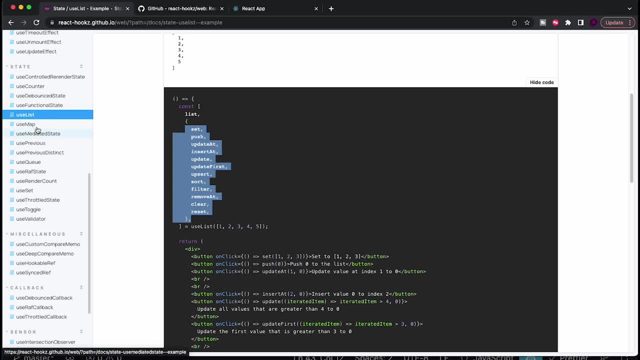 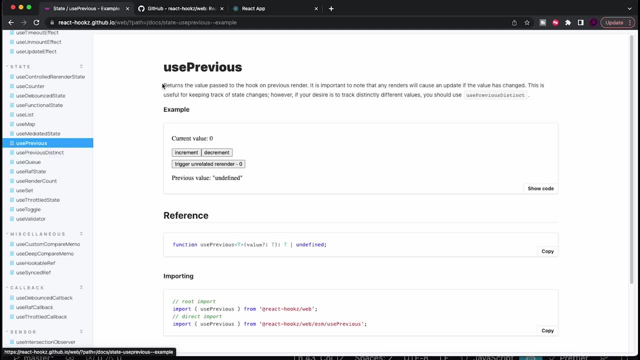 that are built in for that specific list, and they have this not only for lists, but they also have reverse sets, queues and a lot more. I think use previous is also really cool because, as it says, it says it returns the Valley pass to the hook on the previous render and, uh, this I found myself in. 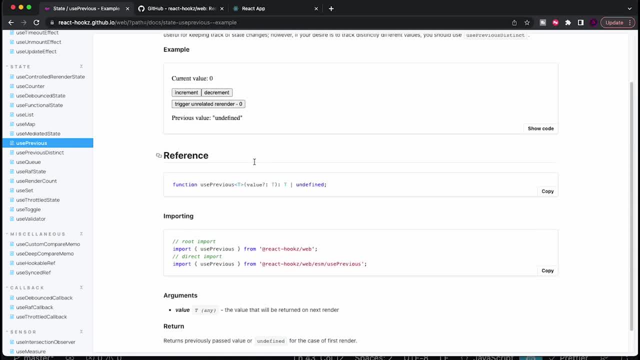 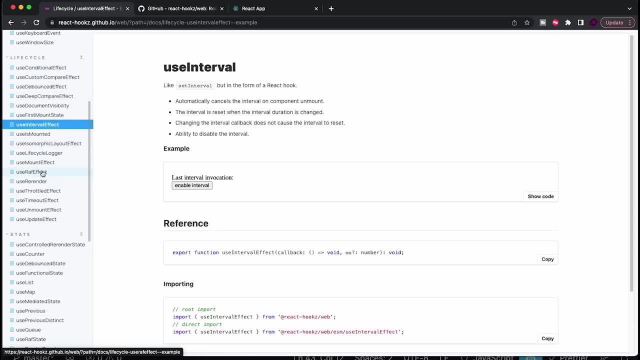 the description is needing, so I think it's definitely useful to shout it out, not to mention all of the life cycle hooks that they also include that if you find yourself, I want to use any of them other than the use the bounced effect, like I showed. uh, you can just come over here and check. 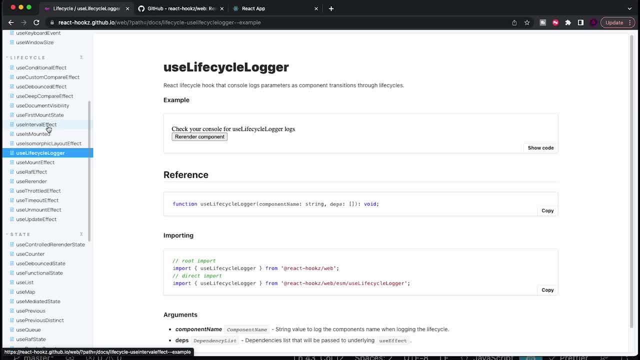 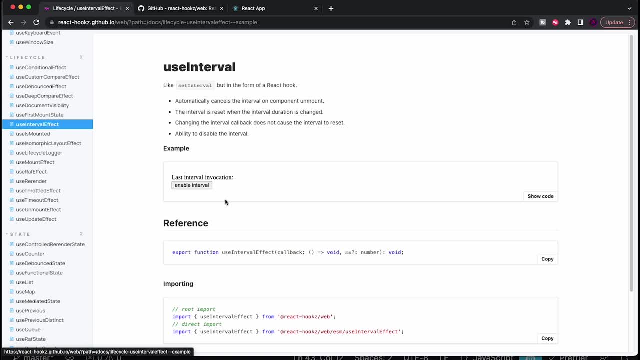 it out. I'll put a link to this uh documentation in the description. but yeah, this is basically it. I really appreciate you guys sticking around for this video. like I said in my post, in my community I'm going to be posting at least twice a week, no exceptions, and this was just a quick video that I 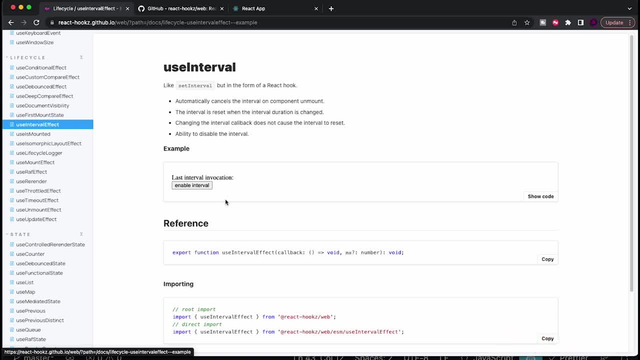 make, because I've been using this library and I just thought, okay, let's just show, show this library to the people. um, if you enjoyed, if you have any opinions, let me know. if there's something I actually should know about this library that I don't know and I didn't mention, let me know in. 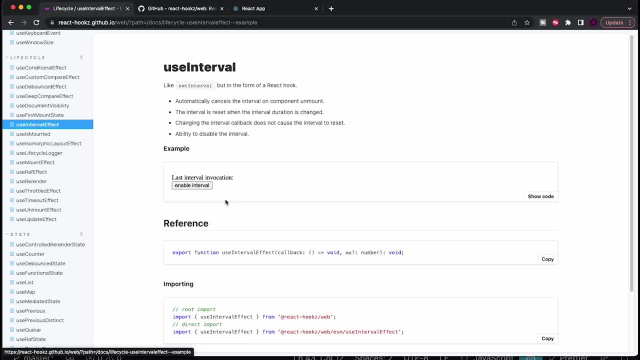 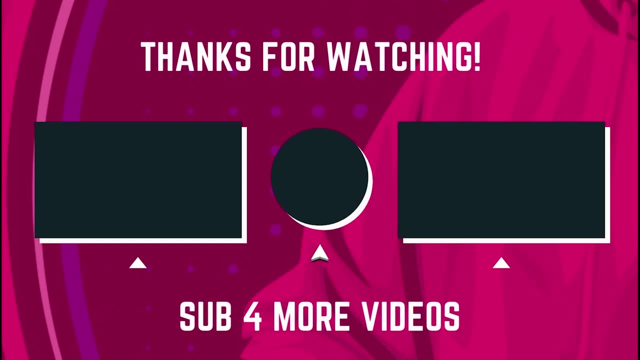 the description. but yeah, that's basically it. I really hope you guys enjoyed it and I see you guys next time.